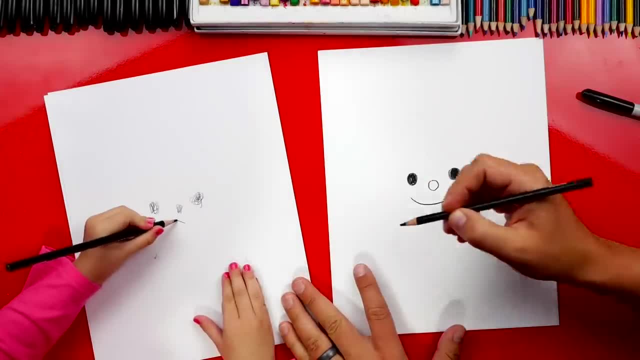 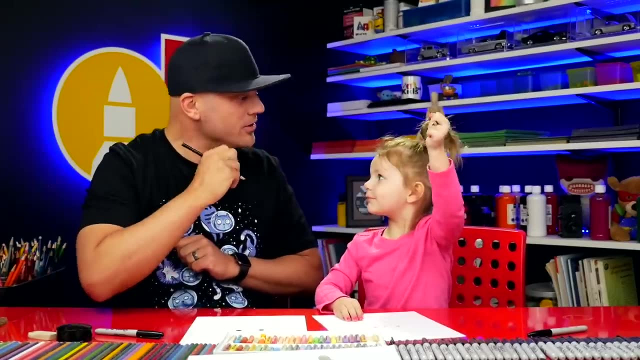 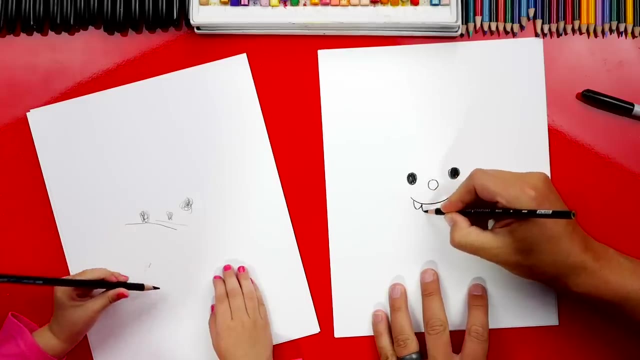 Smile underneath, right here, right underneath the nose. You did it, you did a smile, you did a mouth underneath the eyes and the nose. Oh, should we do the teeth? Okay, we could do the teeth like this on the mouth. do it right here, Yeah. 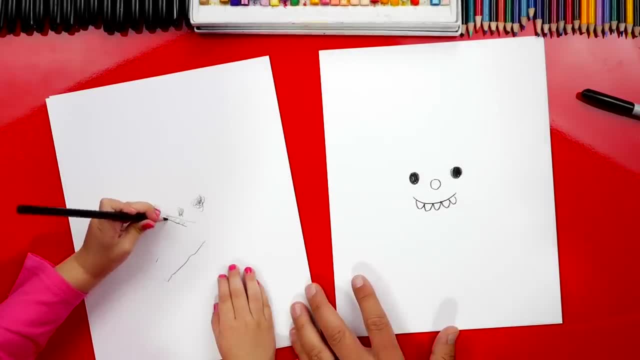 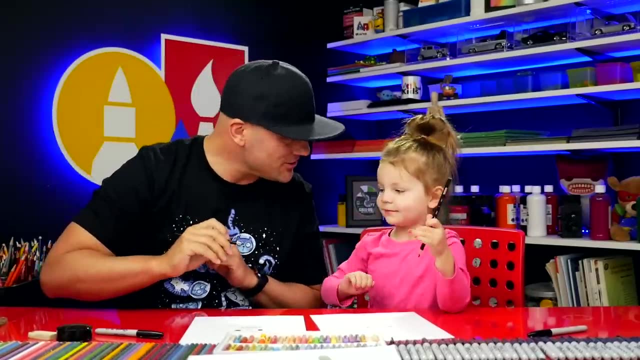 So right there on the mouth, There you go. You did the teeth. good job can be fun. Okay, now let's draw the head. We're gonna draw a. yeah, we're gonna draw a big. watch me, We're gonna draw a big circle around. 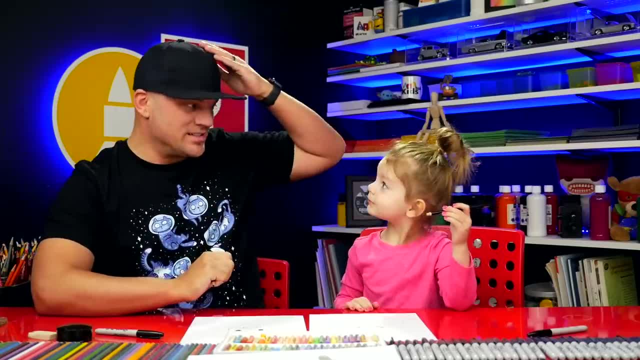 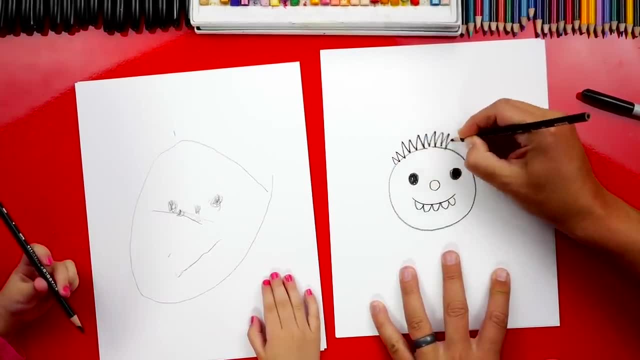 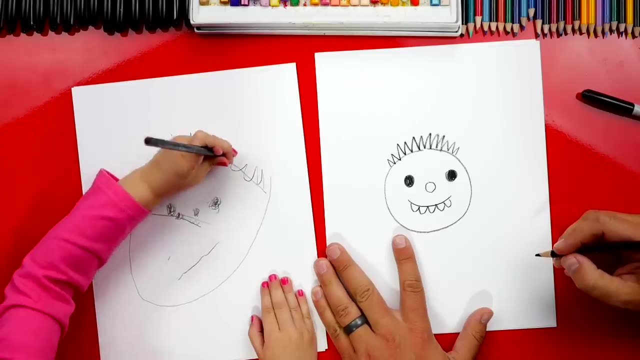 Oh, Okay now what's on top? What's right here? hair. Okay, let's draw some hair. We're gonna draw a zigzag line on top of our head. Can you draw a zigzag line up here on the? for the hair, hair, lots of hair. keep going, Tom more. 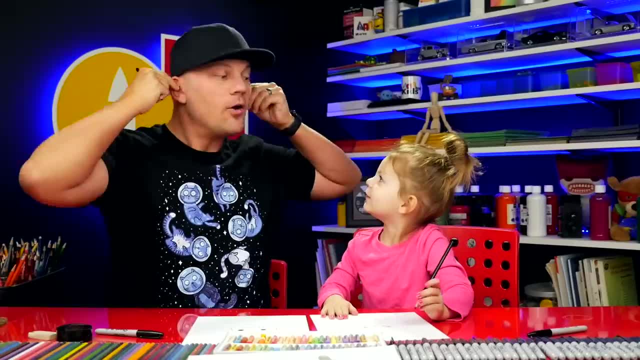 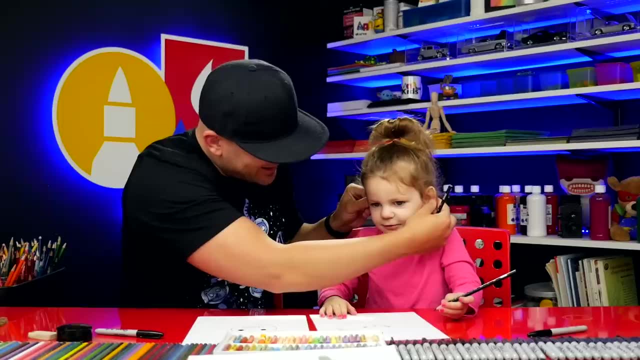 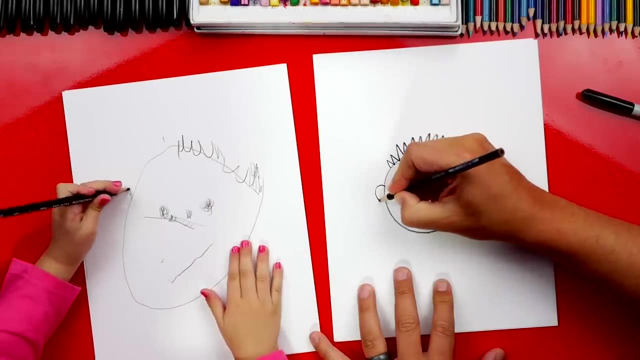 Give me another five. Now let's draw these. what's this called? ears, ears, Yeah, how many ears you have? one, two, Okay, watch me Another one. Yeah, Okay, over here We're gonna draw an ear. Yes, We've been practicing. you know where the ears are. 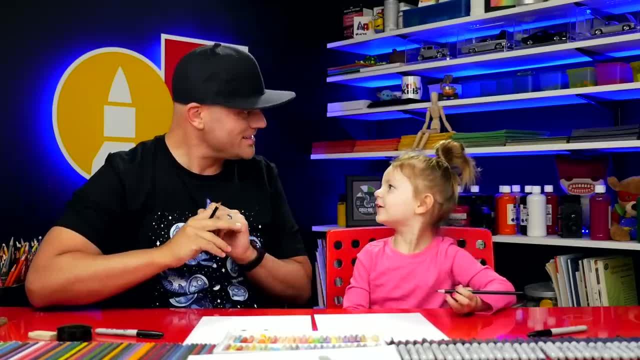 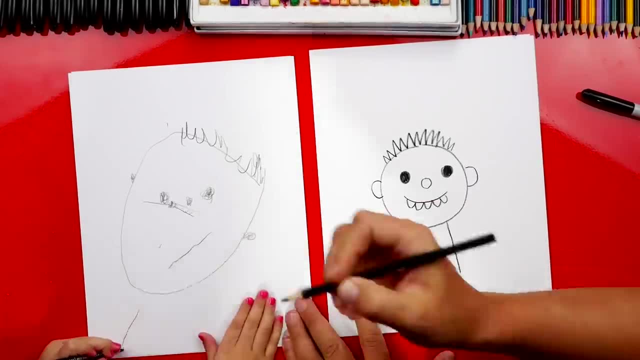 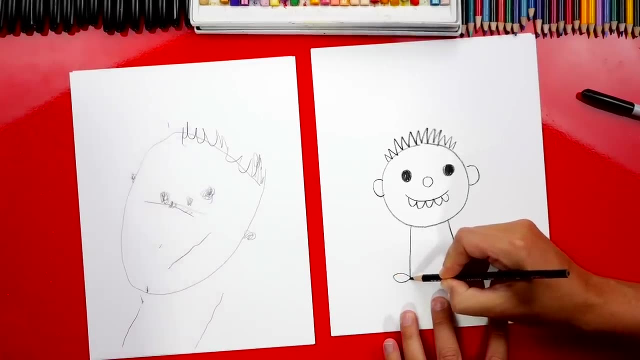 Good job, Olivia. Should we draw the legs and the body? now, let's, let's draw the legs. so we're gonna draw two lines like this: yeah, your turn. there, you go one more. now let's draw the feet. yeah, let's draw. yeah, your feet are on the bottom of your legs. draw a circle right here on the bottom for a. 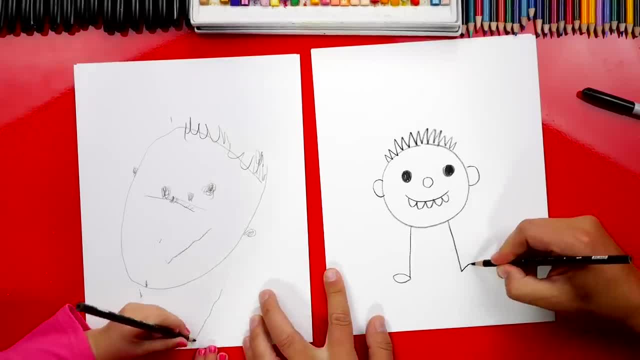 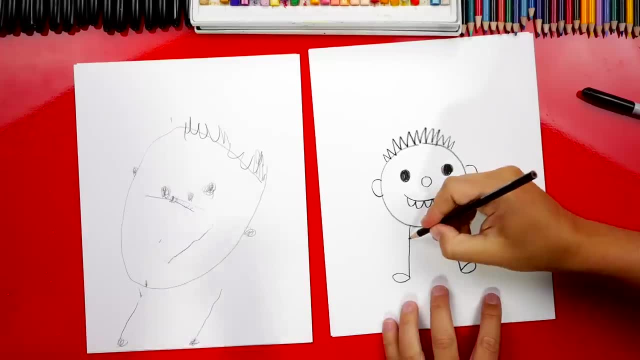 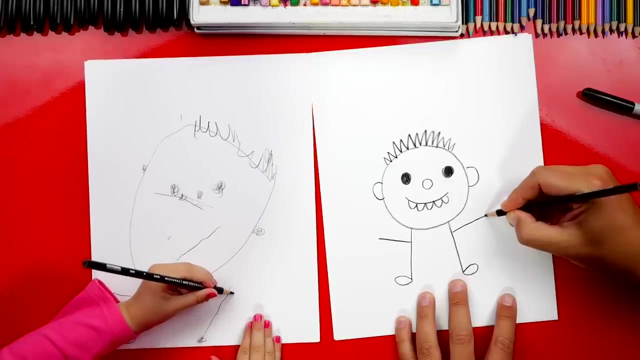 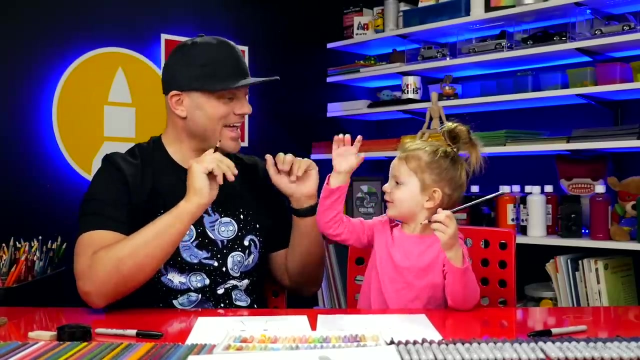 foot, hold your paper. there you go, and let's draw another foot on the other leg, yeah, okay. what are these called arms? yeah, let's draw an arm, one right here, draw a line, yes, and then let's draw another on the other side. what are these called fingers, fingers and hands? let's draw a circle. 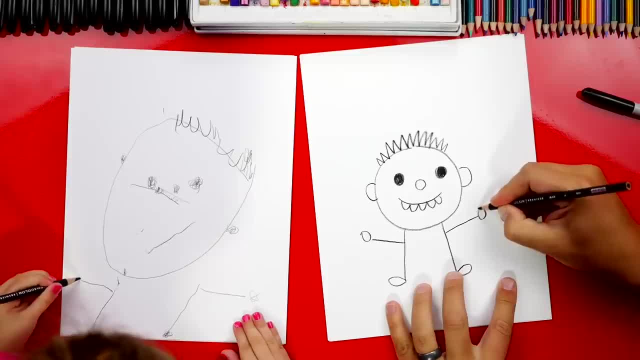 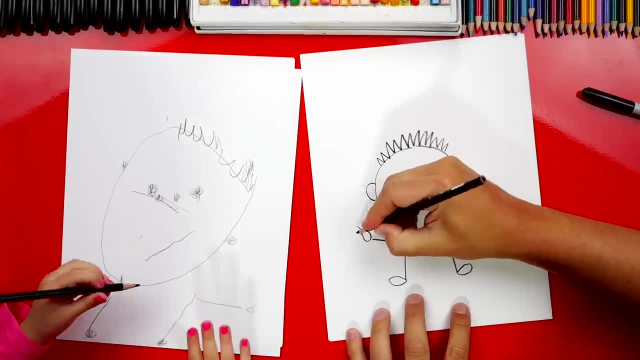 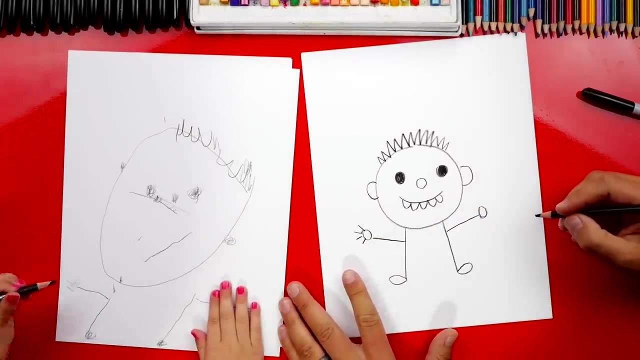 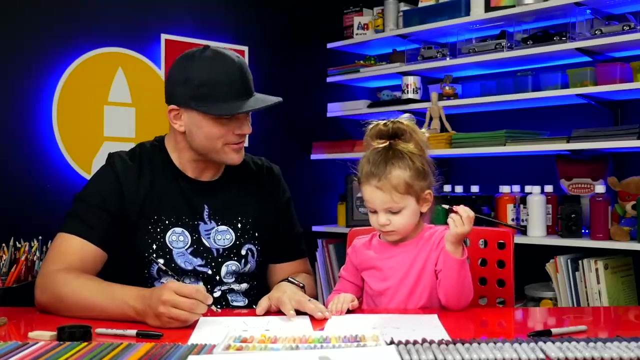 circle right there, and let's draw a circle over here, yeah. and then let's draw the fingers. fingers on our hands, so let's draw lines on our feet, on our hands right here. draw some lines- yeah, good job. and then fingers on the other hand. oh, those are the best fingers ever. 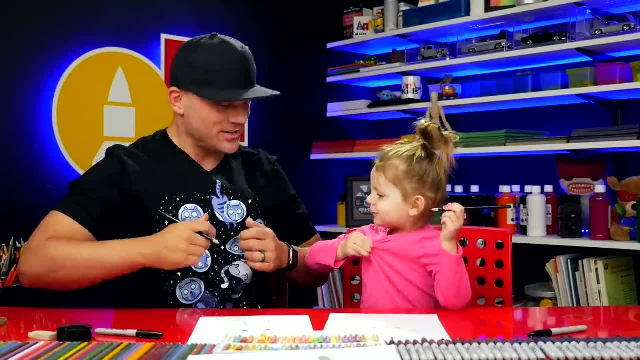 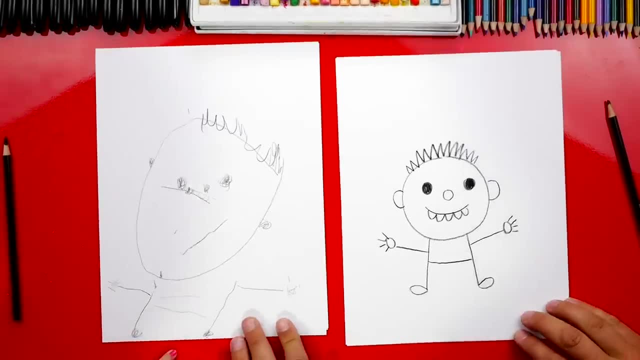 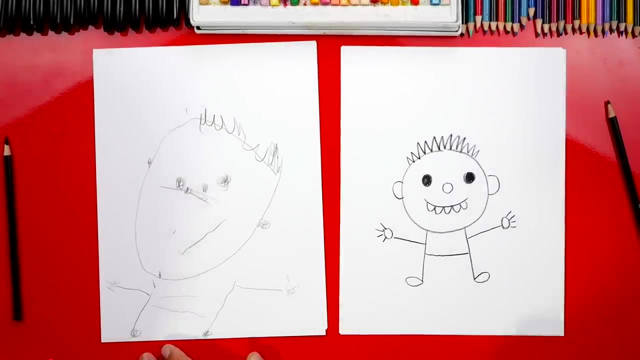 okay, livy, what's this called a shirt? let's draw a shirt on our person right here. yeah, okay, livy, we did it. we finished drawing our little people and yours is perfect. i love that little head. you did such a great job. now we still need to do one last thing. we need to color our 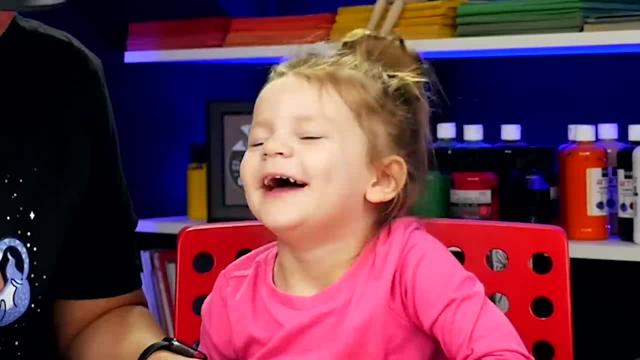 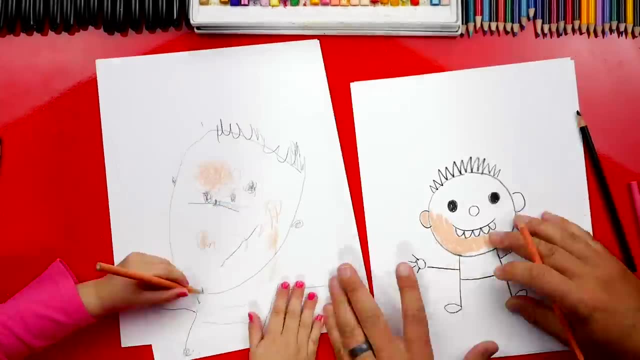 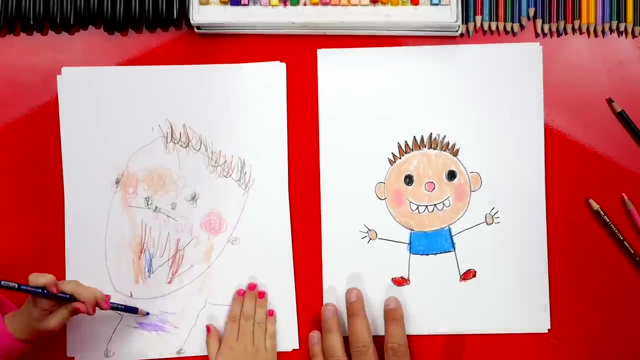 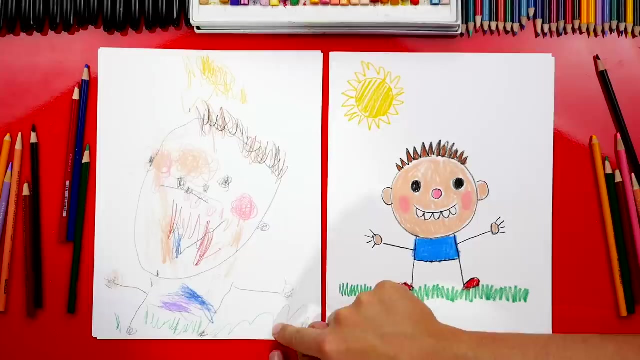 drawings. do you want to color your drawing? yep, okay, this part we're going to fast forward, but you guys at home can pause the video to take time to color your people. now we added some extra things too. what's this down at the bottom? grass, grass, yeah. 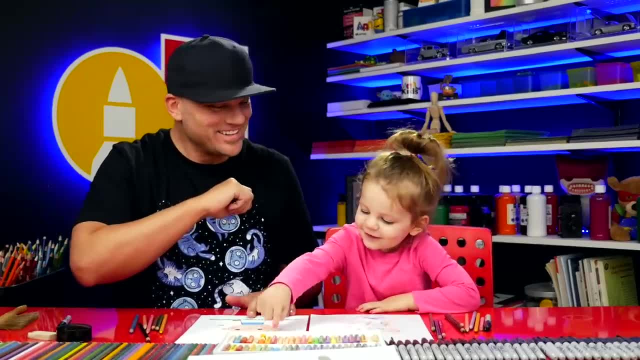 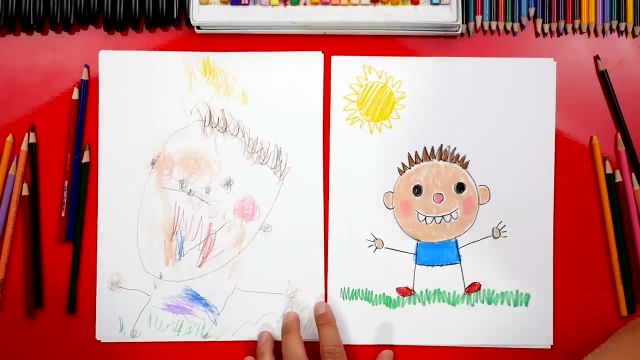 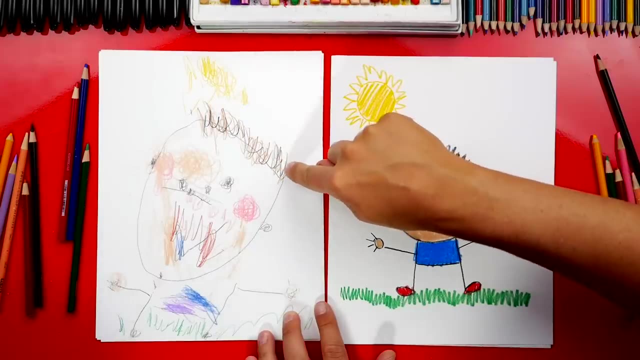 what's this up at the top, a sun livy. what are these called right here? cheeks? yeah, you colored your cheeks pink and you also colored your shirt purple. and what's the color of the hair? yeah, brown. oh, it's brown, yeah. and what color is the grass? 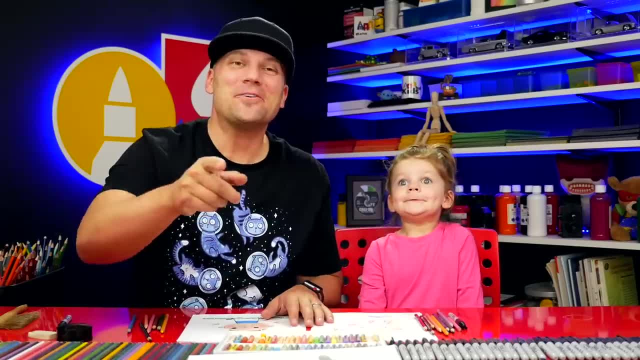 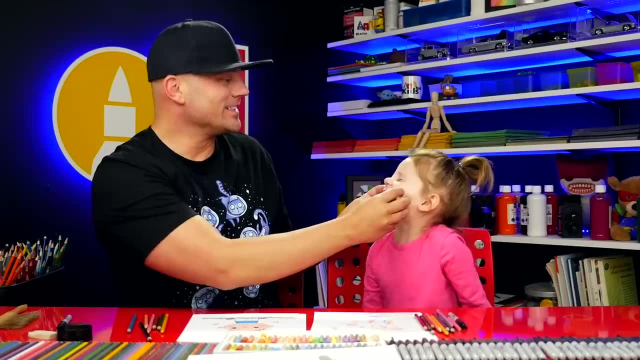 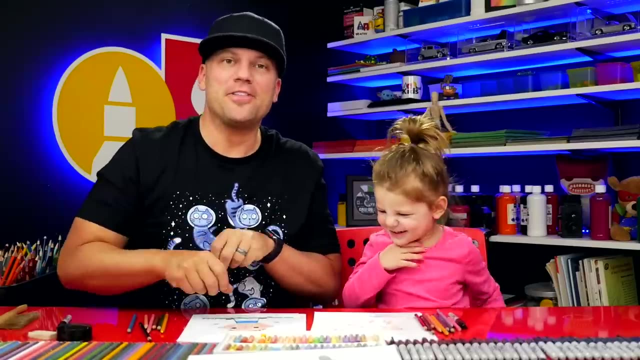 green. you did so great. we hope you guys had a lot of fun drawing people with us, especially our faces, our eyes, our nose. what are these called cheeks? and what's this called neck, neck? also, be sure to challenge your little artist to draw other things in the background. 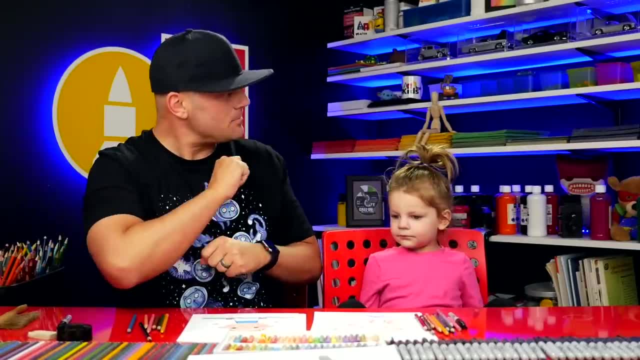 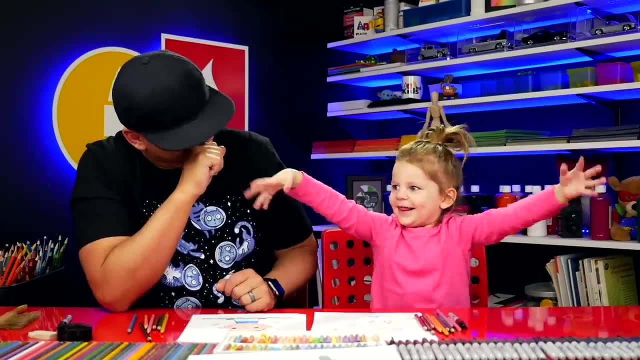 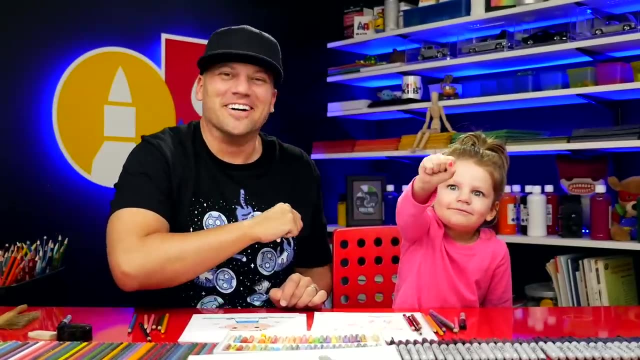 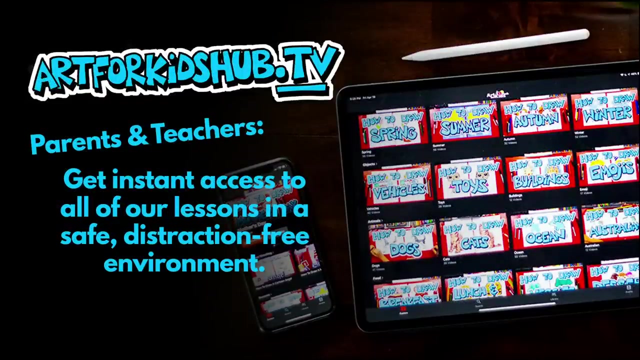 like the sun and grass, maybe some clouds and even some birds. do you like birds? yeah, yeah, yeah, they're flying. let's say goodbye to our art friends. goodbye, do you want to say i love you. i love you, i love you. see you later. goodbye. hey, parents and teachers, did you know that we have an app now for a small monthly price? 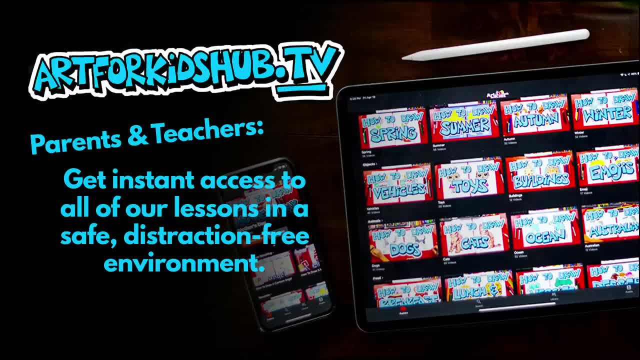 you can get access to all of our lessons in a safe, distraction-free environment. just visit r4kidshubtv to learn more.